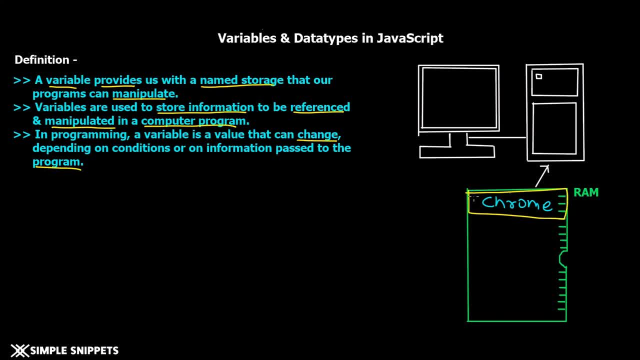 whenever runs in the chrome browser or whenever it is running, it is basically existing in the ram, right? so our ram is basically divided into small, small memory blocks, and each of these memory blocks has some hexadecimal or some binary address, which is pretty weird and long. so you 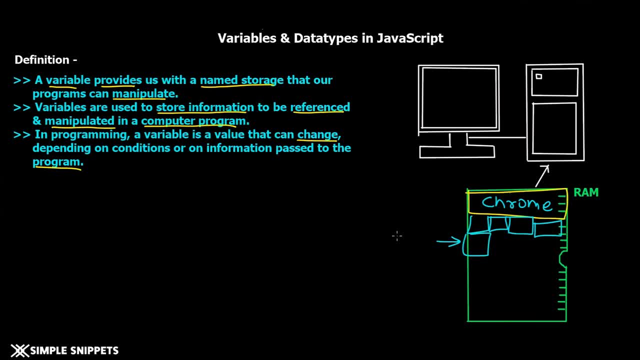 obviously cannot remember as a human being. so it's some hexadecimal values also, like ff, 0x and something like that. so when you create a variable, what happens is in the memory. you allocate some portion of the memory and you give it a name. okay, so that's why we have a named storage over here. so 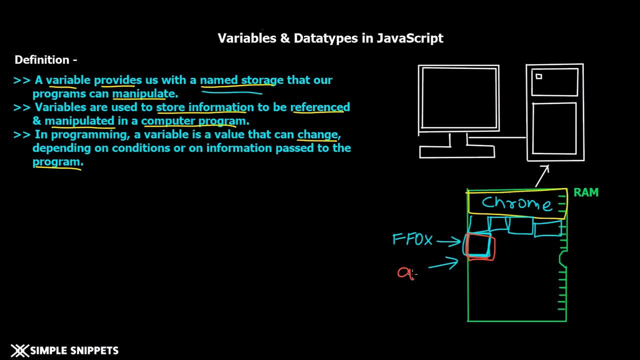 we allocate this memory and we say, okay, i'm gonna name it a. so, even though it has an address which is very weird to remember, we give an alias name, that is an extra name, and we call it a. so in javascript it goes something like this: we have to say where a, and let's say we are storing a number. 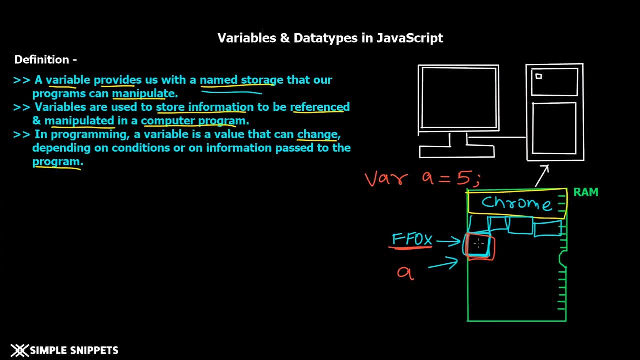 five, okay, and then semicolon. so in this memory block we have the value of five. so we'll talk about the syntax when we actually get into the practical part. but here's what the scenario is now. the next obvious question that you must be having is: why variables? why do we need variables? 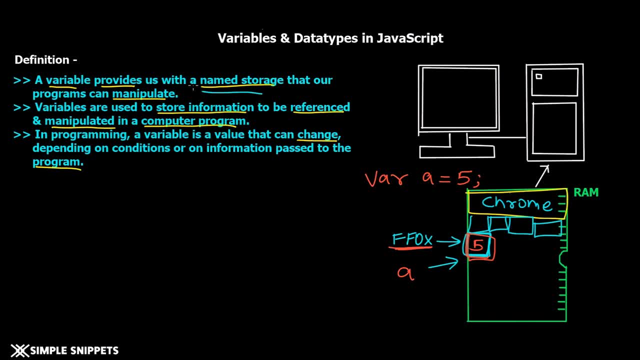 right. so the most simple answer to this is to store data. that's the most simple way i can answer you why you need variables. now imagine a program wherein you are taking values from users of a rectangle, so you're taking length and breadth and your program is calculating the area of rectangle. 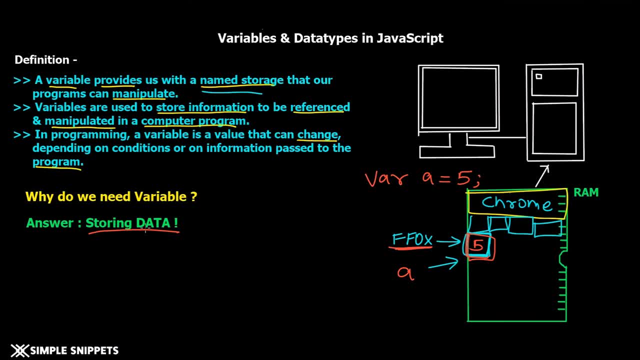 so when you take those values of length and breadth, you need to store them in certain variables, because you want to perform some mathematical operations, right? you have a formula to calculate the area of rectangle, so you'll require some variables. now, obviously, as a human being, you cannot remember each and every memory address, right? so you cannot remember these numbers. so 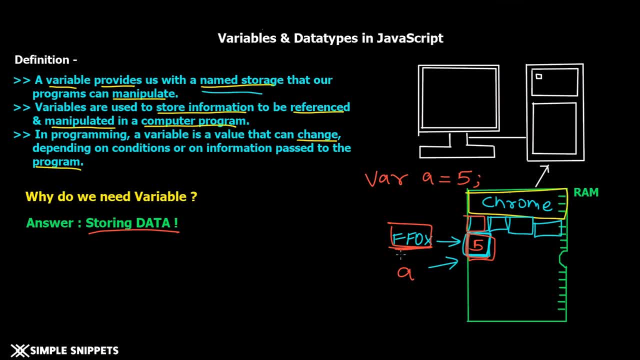 these memory addresses are big numbers which only a machine can read. so this variable helps us by giving it- that memory block, another name, and then we can use this name to access that same memory block. okay, so this is a basic explanation of variables. now let's move on to the types of. 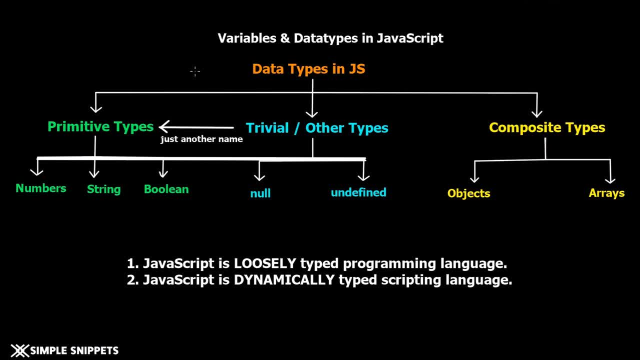 variables or data types of variables. in javascript, the concept of variables: every variable will have a type and basically type means what kind of data is being stored. so, variable, where a can store a number, let's say it's five, it can probably store a string which will have some name abc, and it can store boolean and so on and so forth. so of course, 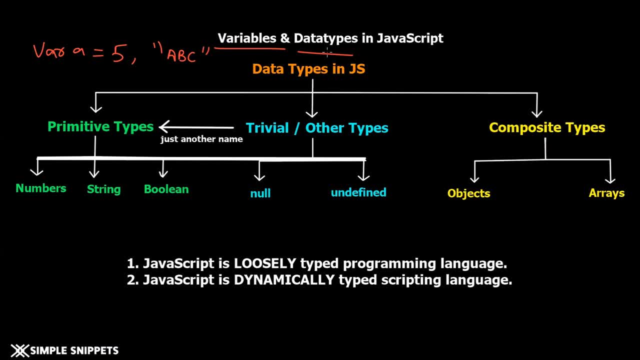 every programming will have a set of data types which are unique to them. so, since we are dealing with javascript, we have these many data types, as you can see in the tree structure. so we have three different types of primitive data types: number, string and boolean. then we have some other. 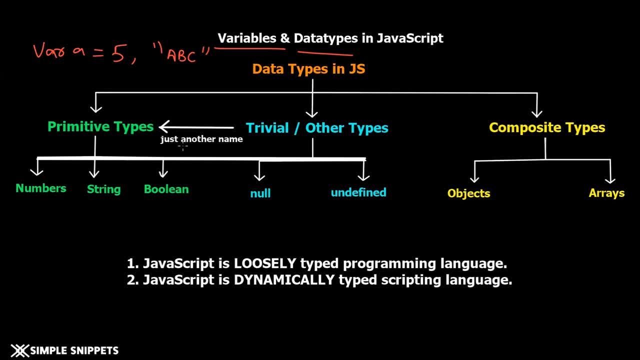 data types, or trivial data types, which are actually primitive, only just that they have one more name, that is trivial, or other types, which is null and undefined. so this is one, two and three. so we have numbers, we have strings and we have boolean as primitive types. again, we have null and undefined. 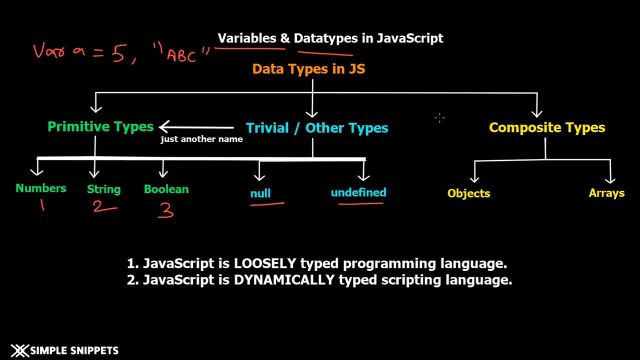 also as primitive types, but they are also called trivial or other types. and lastly, we have composite types, which are complex types basically, which consist of objects and attributes arrays. so we will talk about complex or composite types in further videos, wherein i'll have separate videos for each of these type. right now, we'll just deal with these three primitive types. 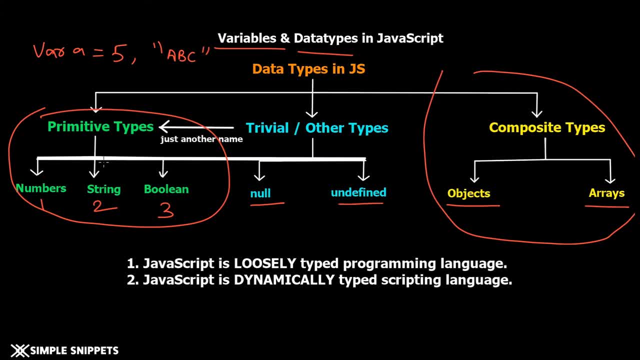 in the programming part. so, before moving to the visual code text editor, that is the practical side. these are two very important points that you need to understand for javascript, specifically for javascript. so let me just read it out and i'll explain to you. so javascript is loosely typed programming language, and the second point says javascript is dynamically typed. 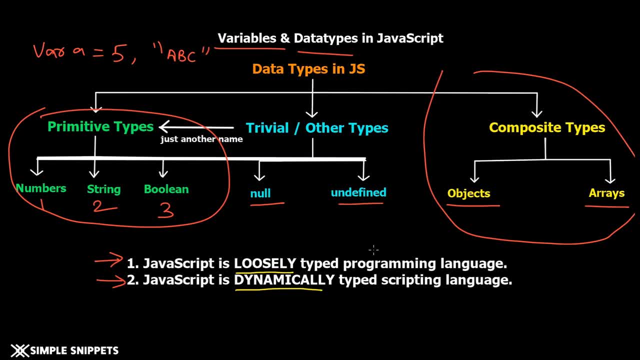 language or programming language. it's one and the same thing, because we are on the client side scripting. now remember these two keywords: loosely and dynamically typed. okay, now let's move on to the programming part, and i'll explain to you what does loosely and dynamically mean, by showing you. 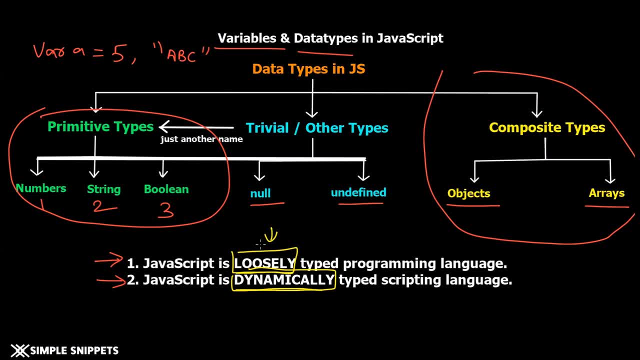 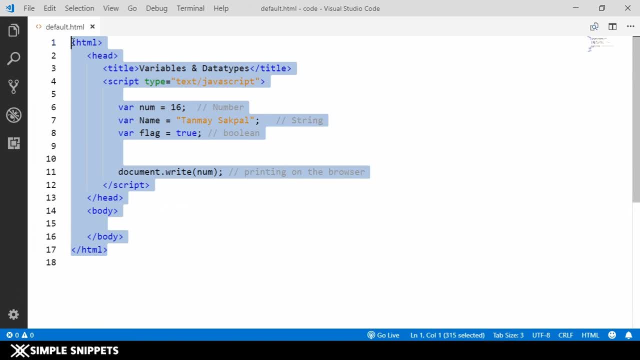 examples, and we'll also see how to create variables and different variations of the primitive types as well. okay, so, as you can see, i have my text editor open. that is visual studio code, and this is our basic html document. inside that we have our script tag. but here we have 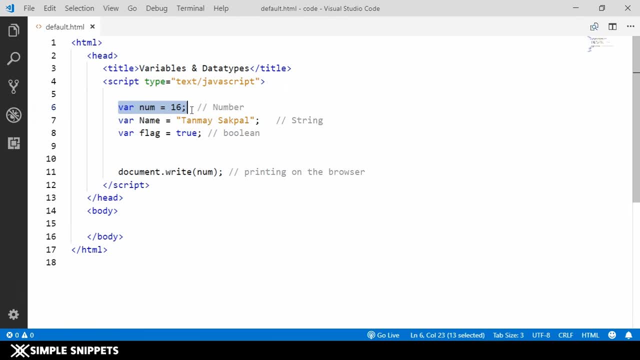 certain variables. so in javascript, this is how you create a variable. now, if you're coming from a c plus plus or java background, this might look a little bit weird to you, right? because in c plus plus and java we used to be like: int x equals to 5 and something like that, right, we we already had. 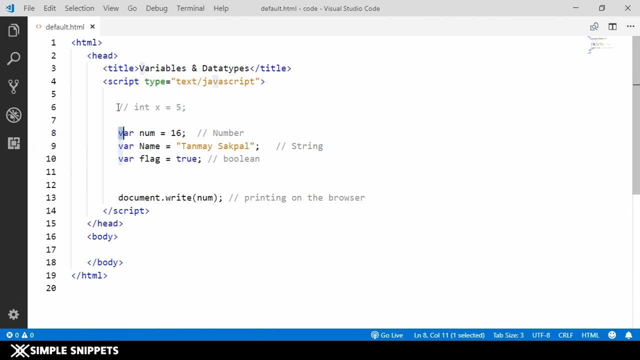 a data type. but here you can see there is no data type. we are only using the keyword var. so this is where that loosely typed keyword comes into picture. that is, js is loosely typed. what this line means is you don't have to define the data type. 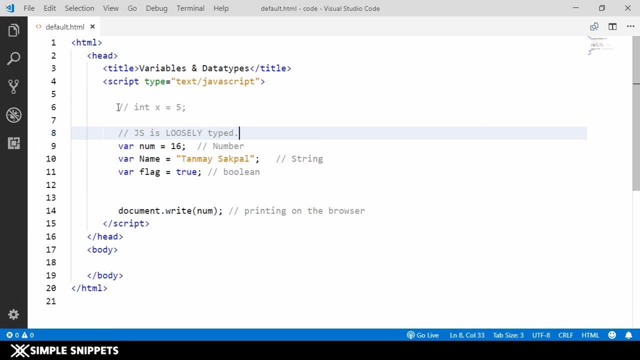 of the variable. when you create the variable, okay, so you don't have to tell what data type it is initially. so what happens is, whatever the type of value you pass in the variable, automatically the data type will change. and this is where the second definition, or second point. 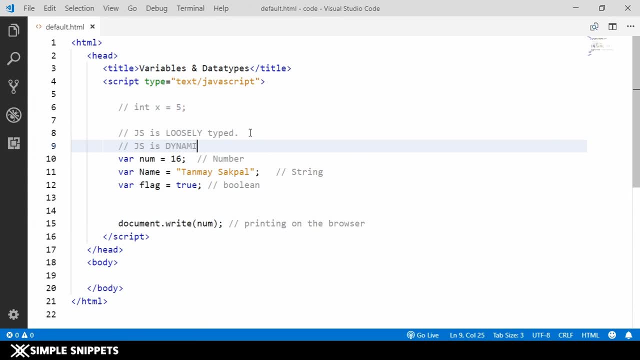 or second property of javascript comes into picture, that is, js is dynamically typed, which means whatever value you pass, depending on the type of value, the data type of the variable will change. now here you can see, we have three different types of variables. so the first one is: 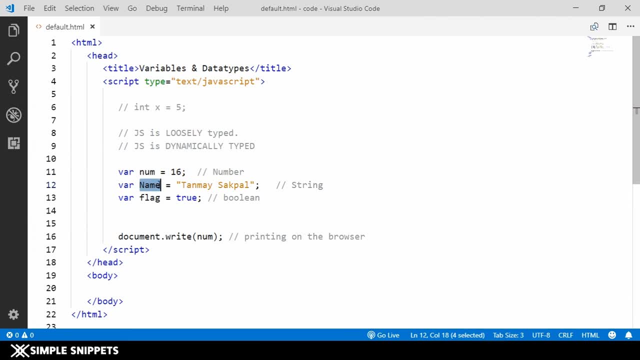 a number type, because we are passing a number in it. second one is a string, because i'm passing a name: tanmay sakpal- yeah, that's my name. and the third one is a flag variable which is having a boolean value which can have two or false, so i can change this to false also. okay, so these are the 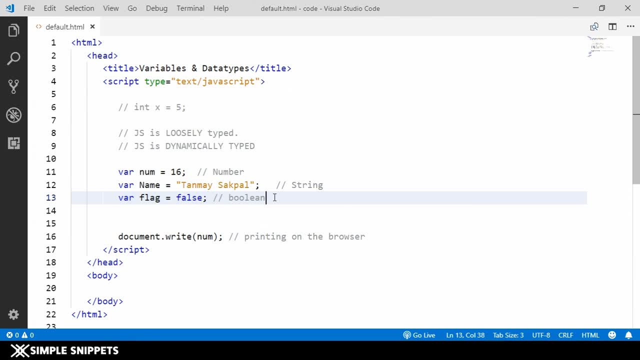 three basic variables, that is, the primitive types that we just saw in the previous digital blackboard. so again, the way you create a variable, you type in var, then you give the name and you can assign a value right there itself, or you can just declare it and later on assign the. 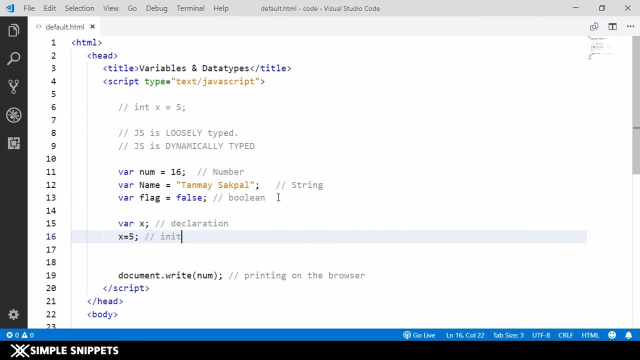 value. so this is just declaration and this is initialization, and you can do both in one single line. you can see, this is that example wherein i've also declared a variable named num and i've initialized the value of 16.. okay, so now, when you're creating variables, there are certain rules. 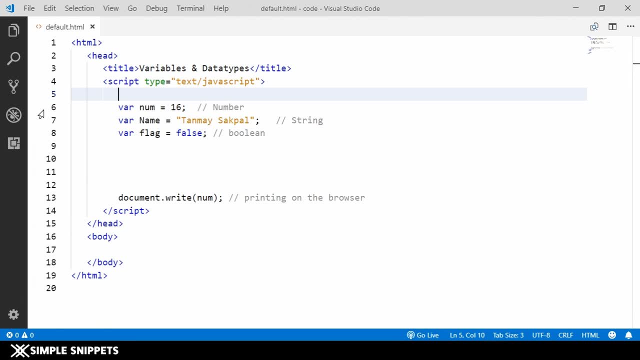 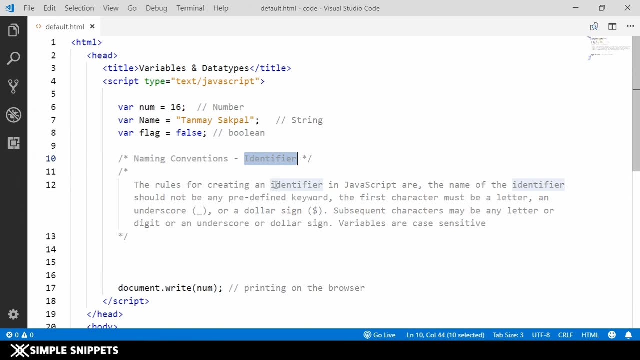 to create variables, that is, to assign names to the variables. okay, so basically what i mean is there are certain naming conventions being followed, which are known as identifiers. so the rules for creating an identifier- basically identifier is the name that you give to a variable in javascript- are as follows. so the 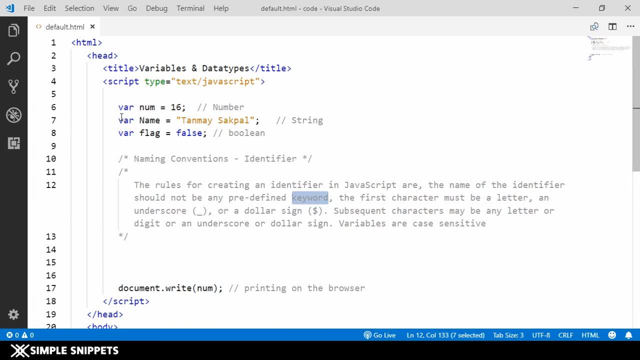 name of the identifier should not be any predefined keyword, so you cannot name your variable as var. okay, so i cannot say var, var. so this is going to give you an error. you can see the error is showing because var is a predefined javascript keyword, so you cannot use that. then the first character must be a letter or an underscore, or. 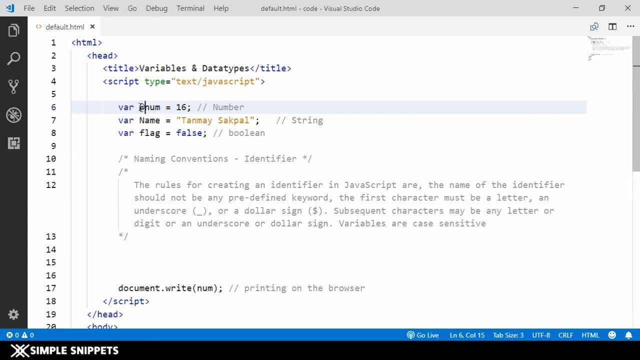 a dollar sign. it cannot be anything else. so i cannot start with var at the rate. so this is again going to be giving me an error. however, i can start off with underscore or a dollar sign, and then the next characters may be any letter or digit or number or underscore as you wish. so you can have. 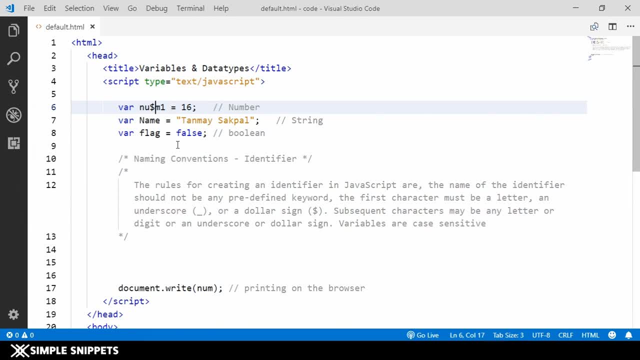 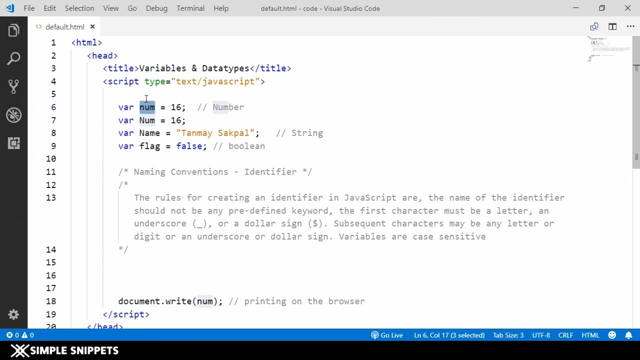 num1 or you can have num dollar, something in between. and lastly, variables are case sensitive, so var num. and if i create one more variable and if i say num where n is capital, then this is different and this is different. so this is what case sensitive means. so there are two different variables. 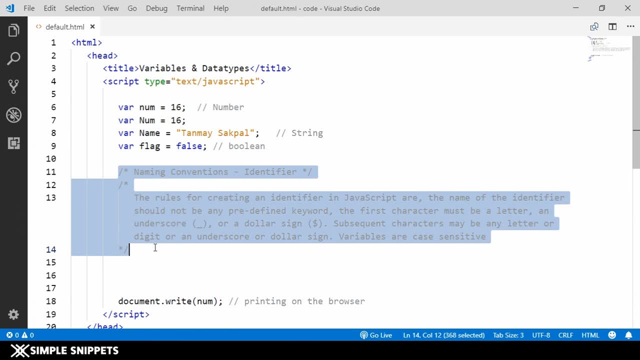 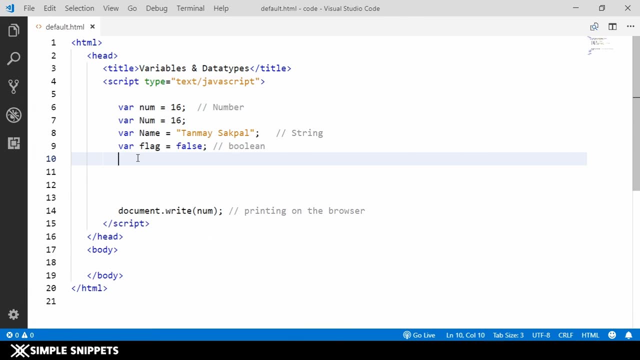 because n is capital. so these are the naming conventions and i hope they are clear in your mind. probably you can write them or note them down, if you're an absolute beginner, or you can just take a screenshot. so, lastly, what i'm going to do is, as you can see, the last statement of this. 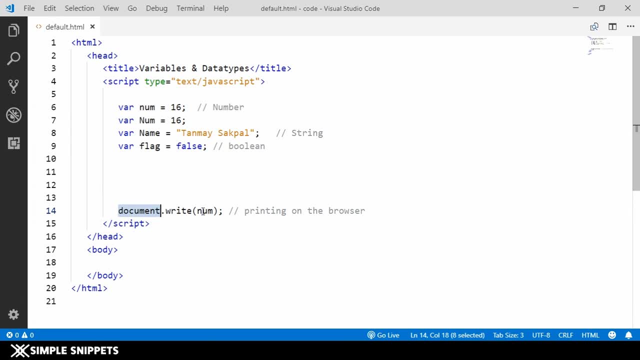 script tag wherein i have a javascript line is document tag dot write num. so what i'm doing is i'm taking this num variable, whose value is 16, and i'm just printing it on the web browser. so let's try to run this defaulthtml, okay? so, as you can see, i just 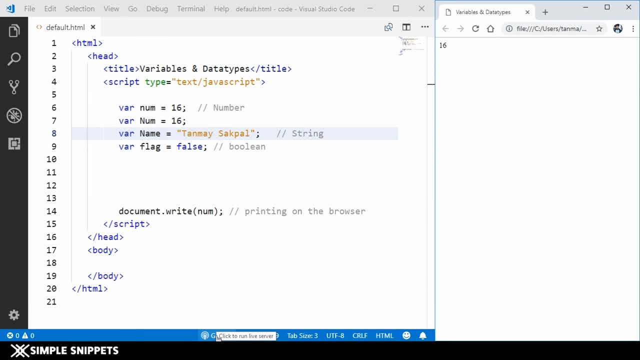 opened that document. i'm not going live as of now. i'm not using the live server plugin, because i just wanted to show you this printing. and then there is another function which you can use, which i just want to introduce over here is the alert function. so inside this alert, i'm just going to 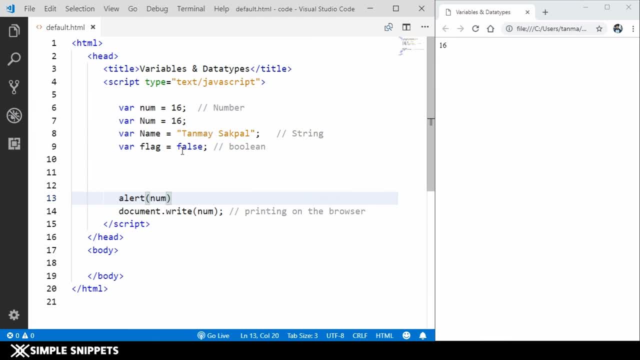 write the alert function. so i'm just going to write the alert function. so inside this alert, i'm just going to write the num and i know i have not talked about functions, but just type along with me. i'm going to comment this documentwrite statement, save this and when i run this, there you go, you can see you. 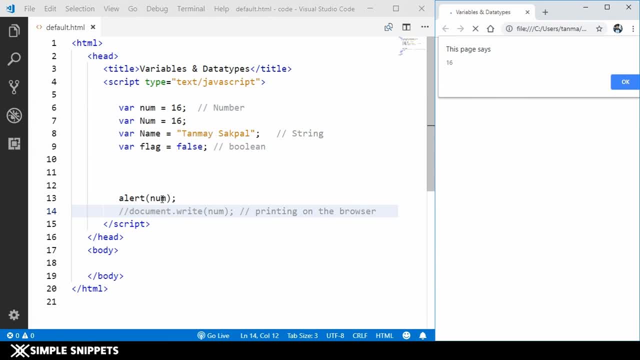 got a pop-up message saying this page says 16.. the 16 is this number variable. i'm just going to say okay, so this is what this function does. so i just wanted to introduce this so that in further videos, when you use it, you feel comfortable. so one more thing that i wanted to show is, as i mentioned, 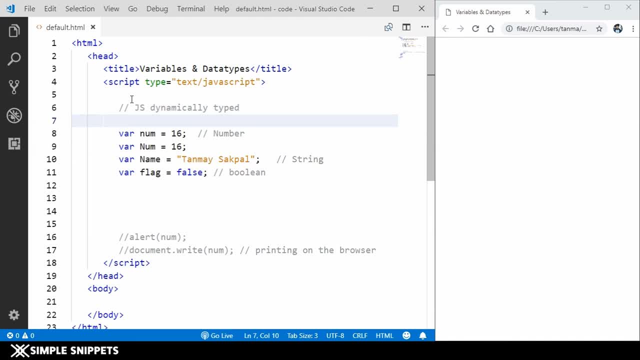 it is dynamically typed, which means the data type of the variable changes depending upon what value you pass. so here you can see. this num is storing 16. that's why it is a number. so what i'm going to do is, at this line, i'm going to say num is equal to, and i'm going to say tanma, which is my name. so now again, 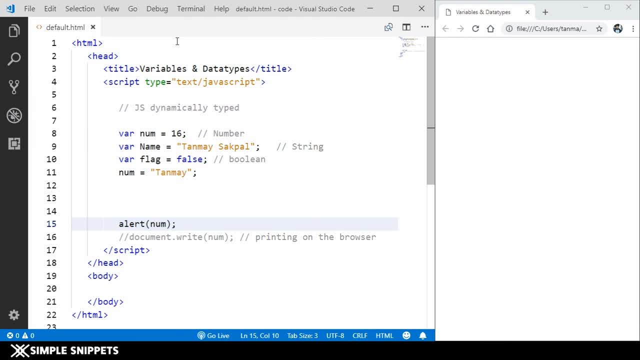 i'm going to just pop up this message in the alert, just save this and refresh this, and there you go. so this is what it is saying. so it's saying that initially our num variable was a number, but at this line- because of course the code runs line by line- at this line the num variable changed its. 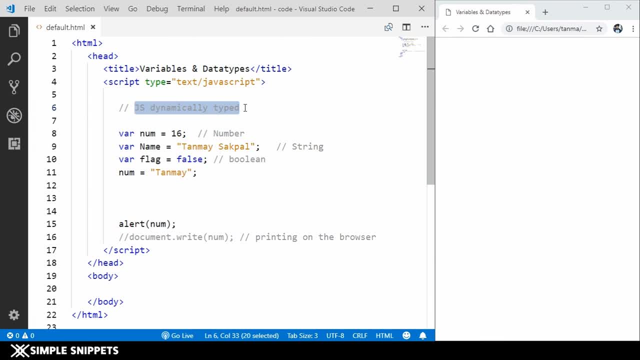 data type to string because we stored a string in it. so this is what is meant by. javascript is dynamically typed, and of course you know what is. javascript is loosely typed right because we don't have to specify the data type initially. we don't have to say int, this will give you an error, so it 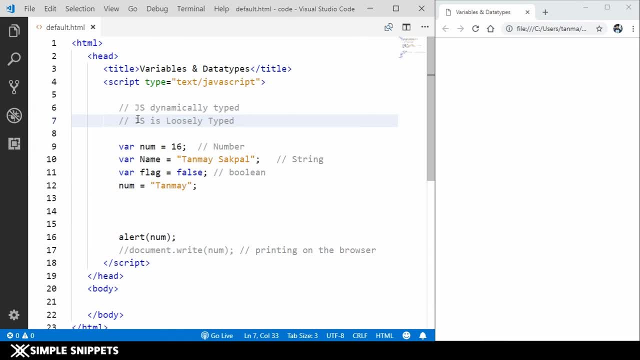 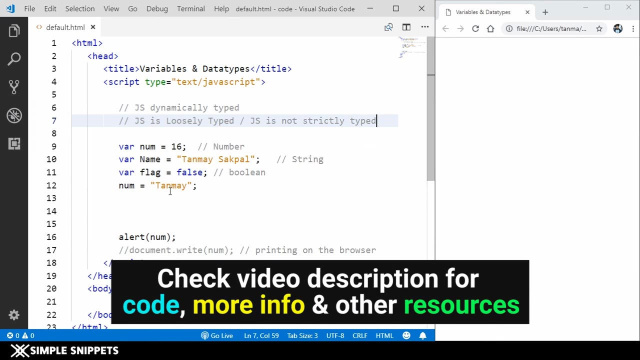 doesn't work in javascript like that. so js is loosely typed. it is. js is not strictly typed. so whenever you see a programming language is strictly typed, it means that the data type or whatever type of data is being stored has to be specified before. so that's it for this video. guys, this was just a basic fundamentals on javascript variables. 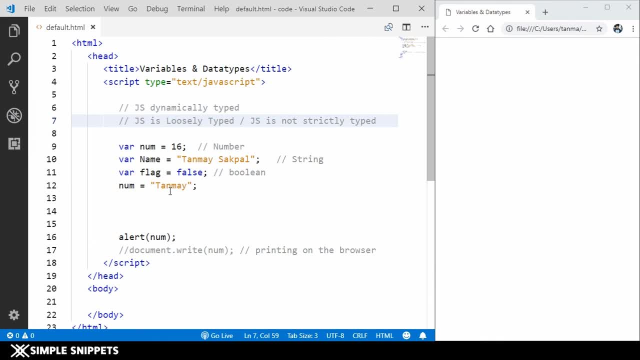 and data types, and i hope you have a good idea about the features. that is, javascript is dynamically and loosely typed, so thanks for watching. guys, if you like this video, please give it a thumbs up. let me know in the comments how this video was. do share it with your. 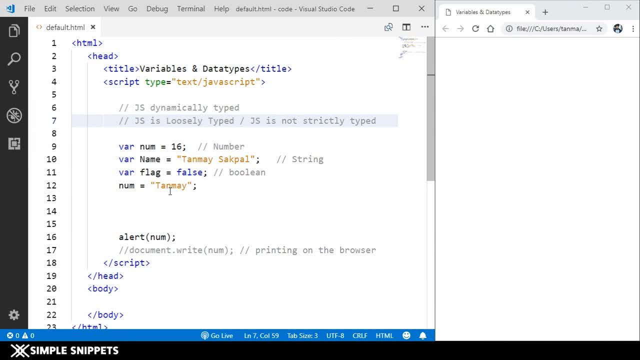 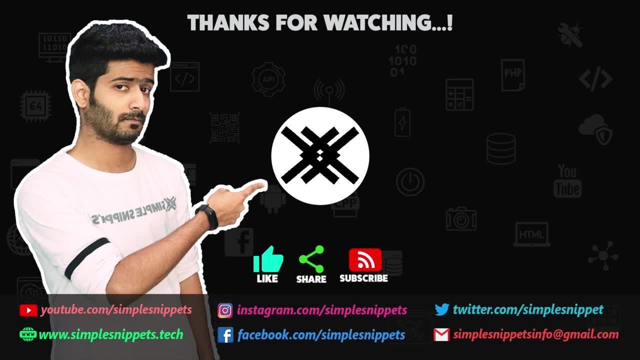 friends, and if you haven't yet subscribed on this channel, make sure you subscribe so that you get notified whenever i upload a new video. so thanks for watching. see you guys in the next video. peace.